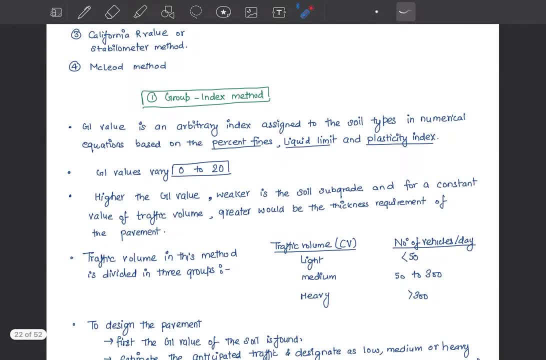 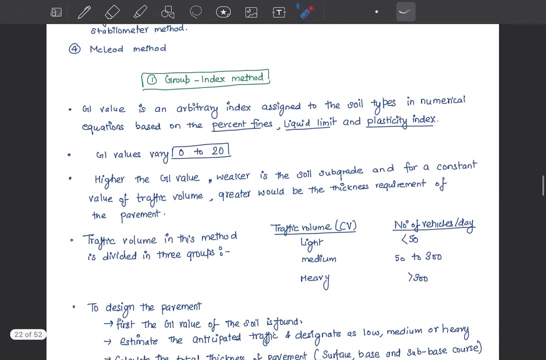 the group index method, which is a type of empirical method. Basically, in the group index method, we used to calculate the GI value first, and on the basis of GI value, the curve has been suggested which recommends the pavement thickness. Okay, so what is GI value? 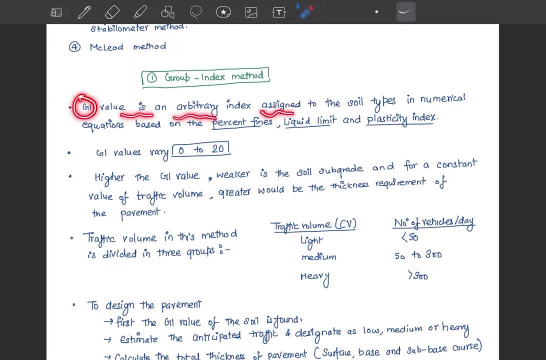 GI value, that is, group index value, is an arbitrary index assigned to the soil types in numerical equations based on the percentage fines, liquid limit and plasticity index. So basically, GI value is an arbitrary index value which we calculate from a numerical equation. 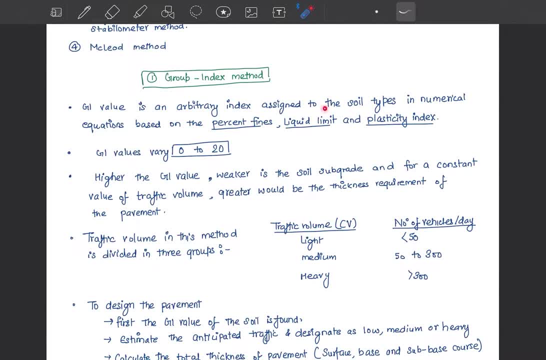 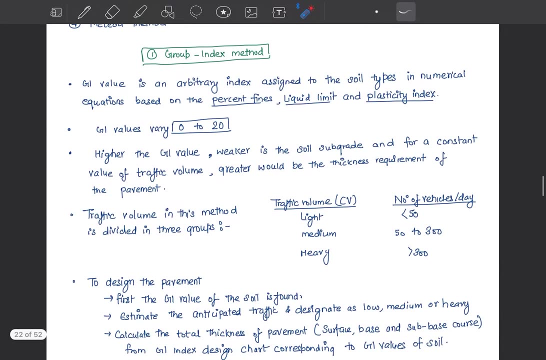 In those equations we need percentage fines, liquid limit and plasticity index. And how do we calculate plasticity index? That is the difference of liquid limit minus plastic limit means we also needed plastic limit. Okay, The group index value varies from 0 to 20.. 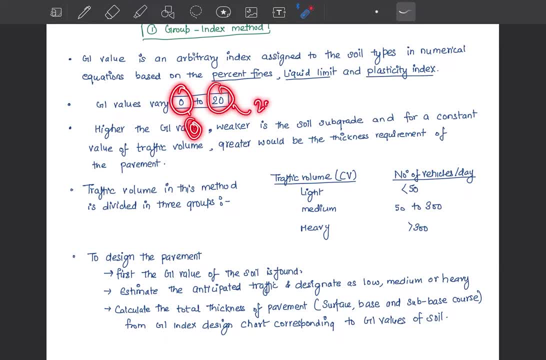 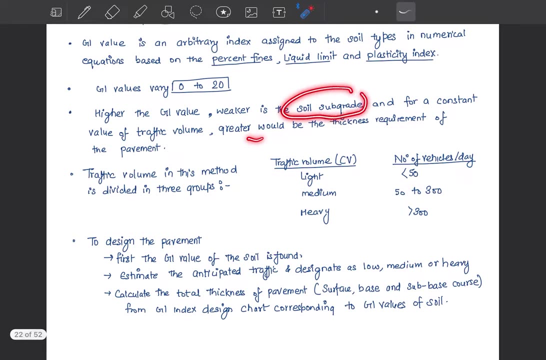 So minimum group index value is 0, and the maximum group index value is 20.. As higher the GI value, the higher the group index value. the weaker the soil subgrade will be Okay And the weaker the soil subgrade. 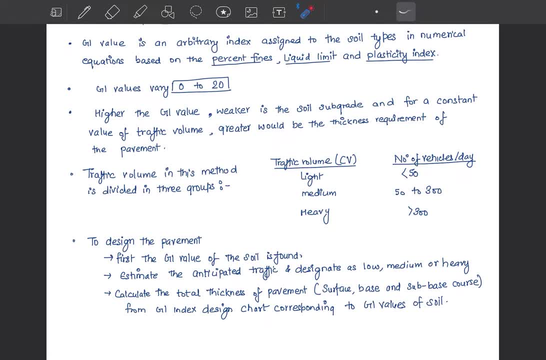 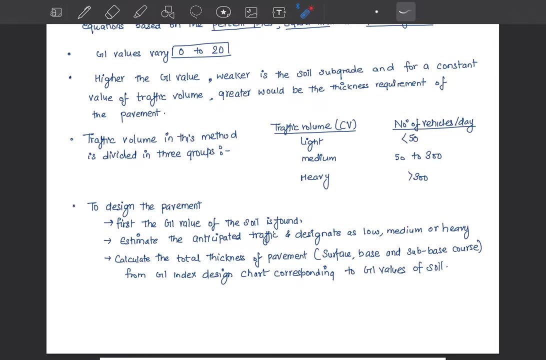 the higher the pavement thickness requirement will be. Okay, Remember, as high as the GI value, weaker would be the soil subgrade and simultaneously, greater would be the thickness requirement of the pavement. Okay, Now, in this GI method, the requirement we have, 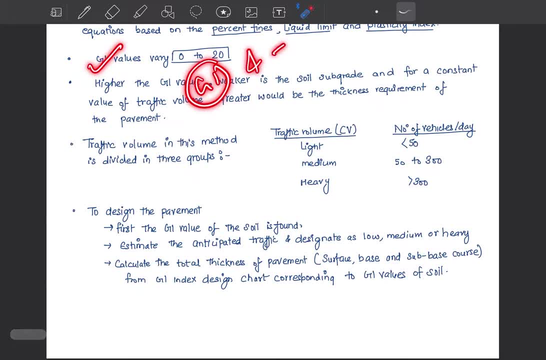 there are two things: One is the requirement of GI value and second is the requirement of your traffic volume. Okay, So traffic volume is basically divided into three parts, divided into three groups: light, medium and heavy traffic. Okay, 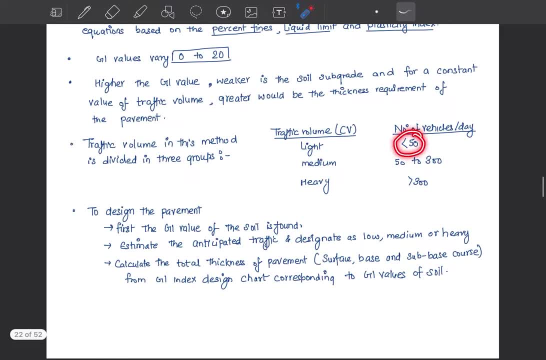 Then on the basis of number of commercial vehicles per day, if 50 is less, then it is classified as light. If it's in the range of 50 to 300, then it is classified as medium And if it is greater than 300,. 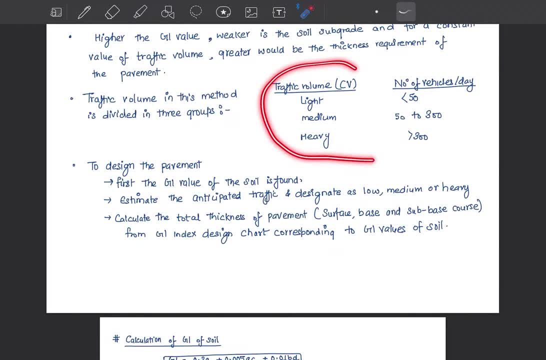 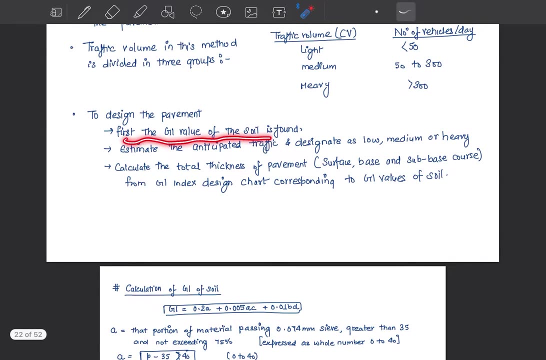 then it is classified as heavy. Okay, So traffic volume has been categorized under the group index method with this following recommendations: Okay, So what are the steps to design the pavement? Looking at the steps to design the pavement, first, the GI value of the soil subgrade is found. 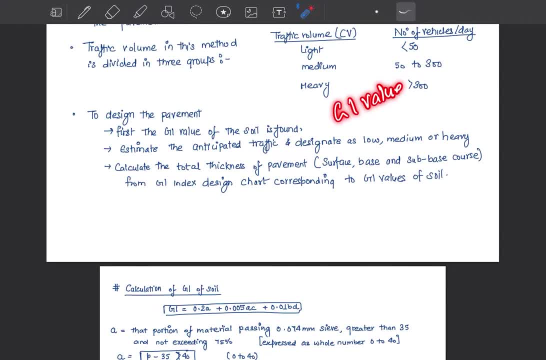 Okay, So the first step is to calculate the GI value. Now, how to calculate the GI value, We will study that in the next step. Okay, The second step is to calculate the GI value. Okay, After that we will find out. 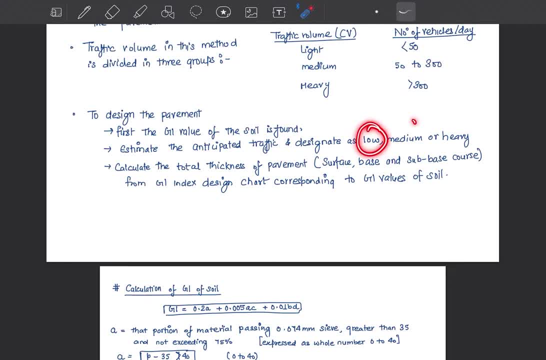 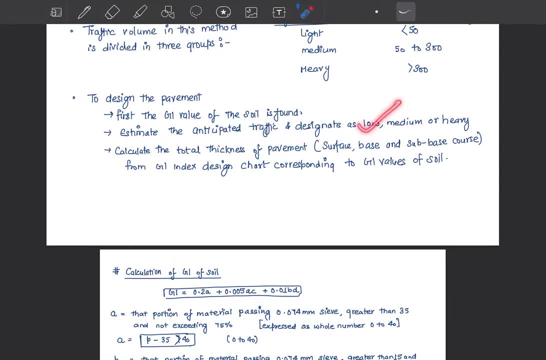 what kind of traffic you have. Okay, Whether it is a low traffic, whether it is a medium traffic or whether it is a heavy traffic. Okay, So first the GI value is calculated. Second, we have to categorize the traffic. 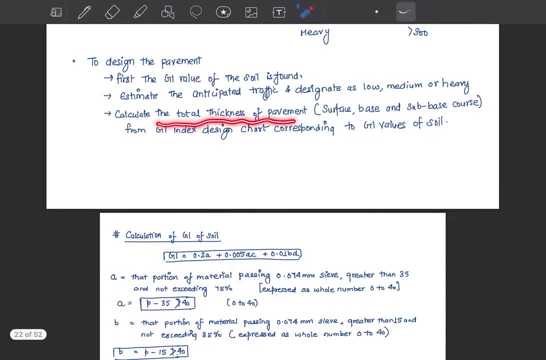 whether it is low, medium or heavy. And thereafter we will calculate the total thickness of the pavement surface base and subbase scores from the GI index design chart corresponding to the GI values of the soil. Okay, When we calculate these two. 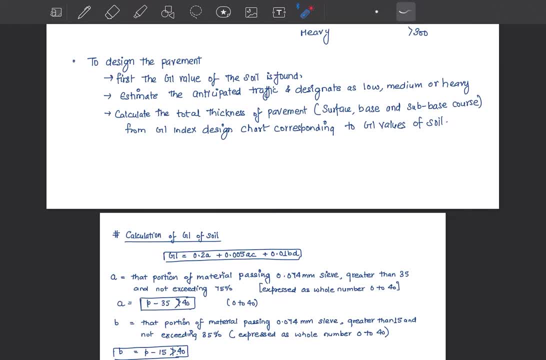 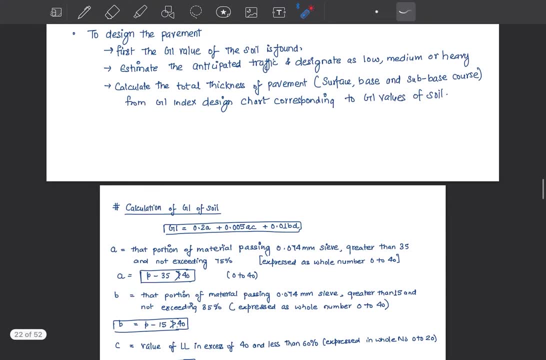 then the design chart of the group index will be given to us. Okay, Simultaneously for the group index values, we will calculate the GI values of the soil. Okay, We will calculate the payment thickness requirement. Okay, Now let's talk about. 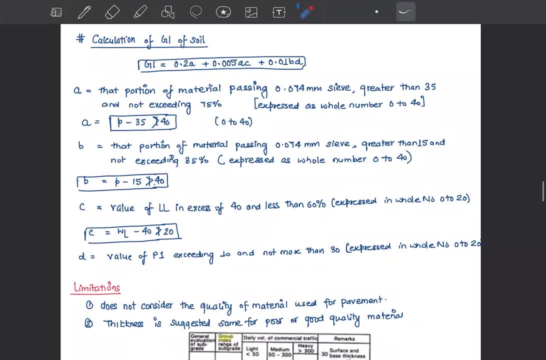 how we will calculate the GI index. Okay, Let's talk about GI value calculation. So the GI formula is that is, 0.2A plus 0.005AC plus 0.01BD. Okay, From this formula we calculate the group index values. 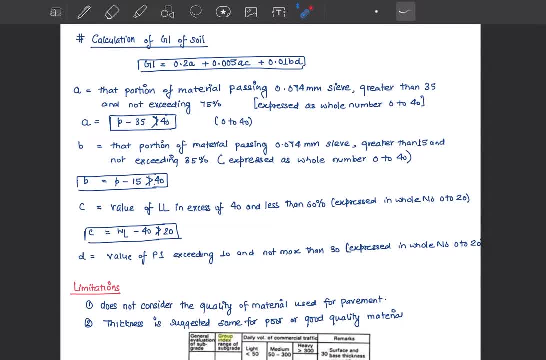 Okay, The group index values is the portion of material passing 0.074 mm sieve greater than 35 and not exceeding 75 percent, and it is expressed as a whole number from 0 to 40. let us say 55 percent of the material is passing through this particular sieve. then can we say like this: 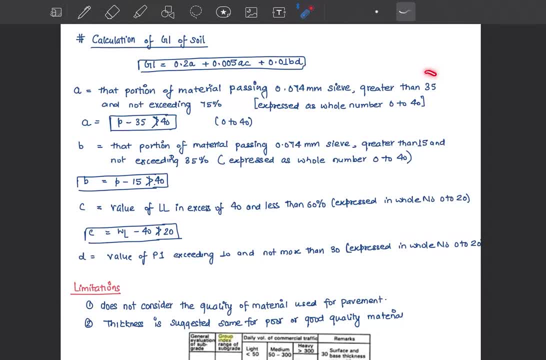 55 minus 35 is around 20, and this should not be greater than 35. okay, sorry, this 55 percent should not be greater than 35 and greater than 35 and should not exceed 75. okay, the path is a. this statements are quite confusing. okay, we have just written it down in the short. 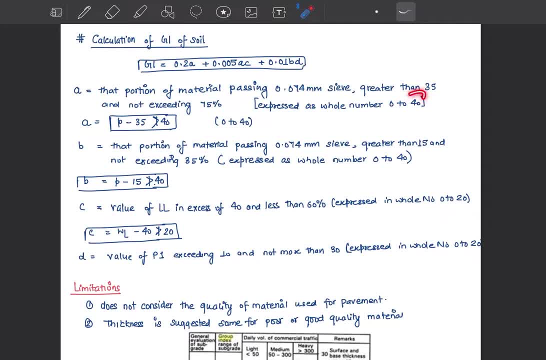 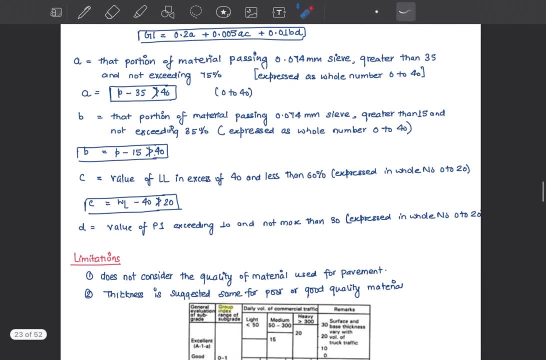 that is, p minus 35, should not be greater than 40. that is expressed maximum up to a whole number of 40. whereas looking at b, that portion of material passing 0.074 mm sieve greater than 15 and not exceeding 35 percent- okay, expressed as same 0 to 40. 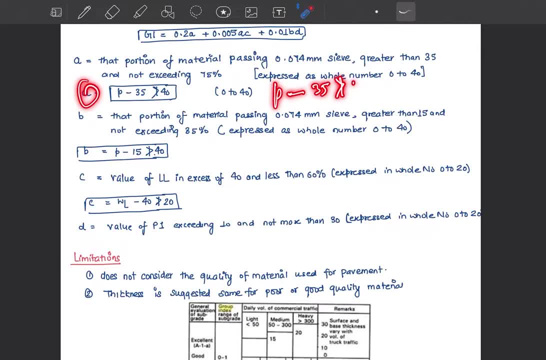 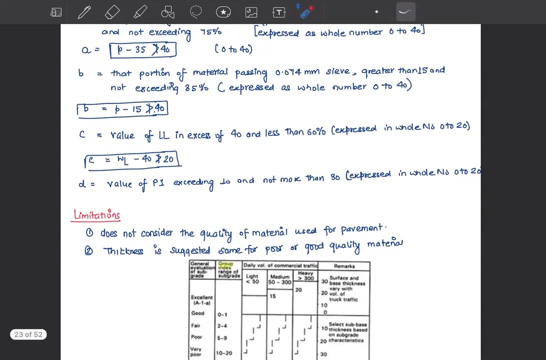 what is a is the portion of material which is passing 0.75 ms greater than 35, but not exceeding 75. and what is b? that portion of material which is passing 0.074 mm sieve greater than 15 and not exceeding 35 percent. okay, what is c? c is the value of liquid. 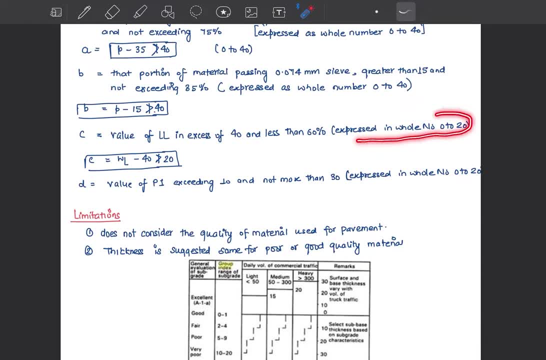 limit in axis of 40 less than 60, and this is expressed in the range of 0 to 20.. so first both were 0 to 40 and the other two are 0 to 20.. ok, the other two will be 0 to 20.. 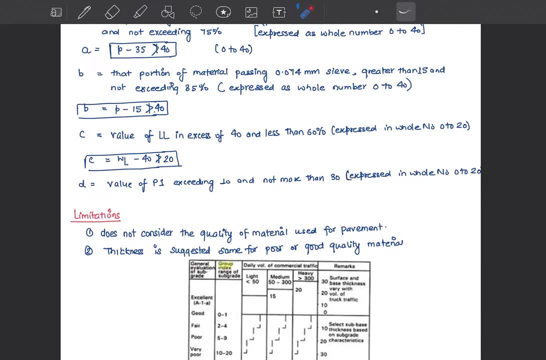 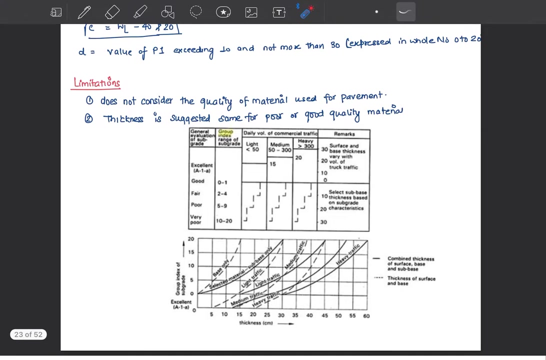 ok, the other two will be 0 to 20.. ok, the other two will be 0 to 20.. so first two were 0 to 20.. ok, and the second two will be 0 to 20.. ok. So C will talk about the liquid limit. D will talk about the plasticity index, that is, value of plasticity index exceeding 10 but not more than 30,. 10 more than 10 but less than 30,. liquid limit more than 40 but less than 60, now A, B, C, D, we will be able to calculate with this expression. now there are certain limitations of this method. what are those limitations? 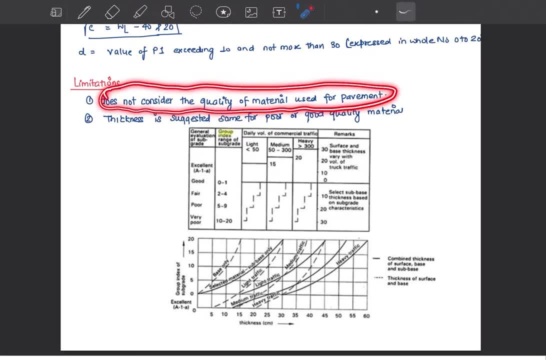 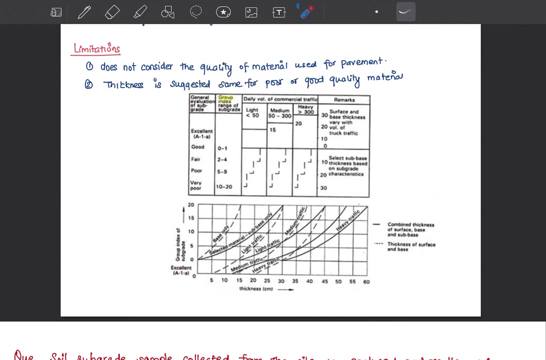 that this does not consider about the quality of the material used for the payment. okay, in this method the material quality is not talked about anywhere. okay, if the material is bad, then also the thickness requirement will be the same. okay, whether it is a poor material or a good quality material, the thickness would be suggested same on the basis of the group index values. what we were discussing about the group index design chart. so this is the group index design chart where you can see 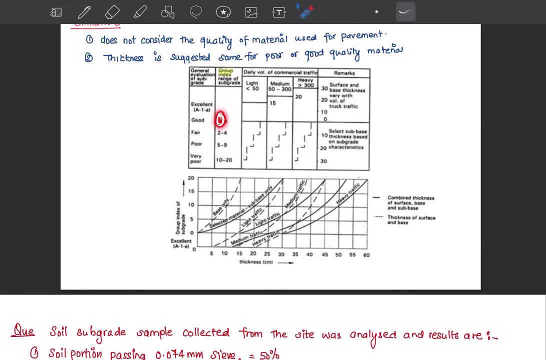 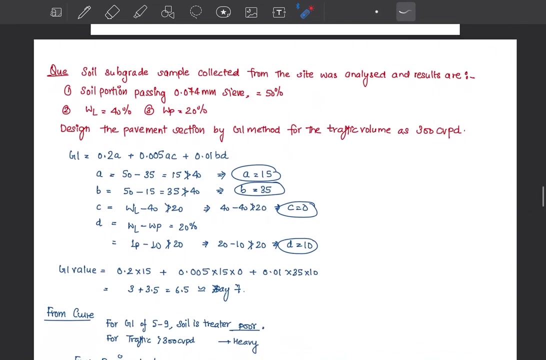 the group index values of the subgrade soil is minimum 0 and maximum 20,, so between 0 to 20, the group index values of the subgrade soil and in light, medium and heavy traffic circumstances, it is given that how much thickness is required. and this is about the combined thickness requirement. okay, now let's solve a numerical to make it more clear about the group index method. okay. now the network unoil has taken a new representation from the site and was analyzed and the results are: the soil portion passing 0.0 modem is C is 50%, the liquid limit is 40%, the plastic limit is 20%. design the payment section by the. 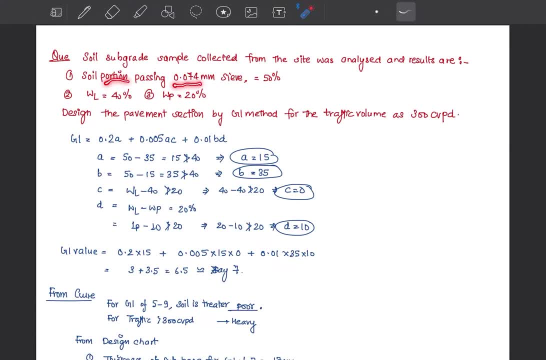 a, a categorization that our traffic is coming in which category. After that we will refer to the GI design chart and from there we will suggest the requirement of the value of the payment thickness. So the first step is to calculate the GI value. What was the GI value? That is 0.2A plus 0.005AC plus 0.01BD. 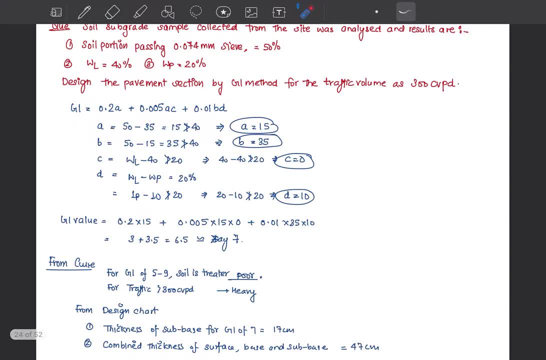 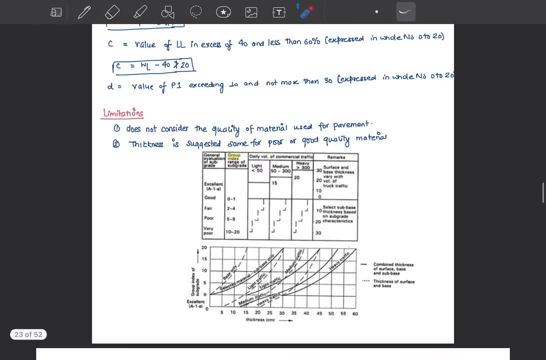 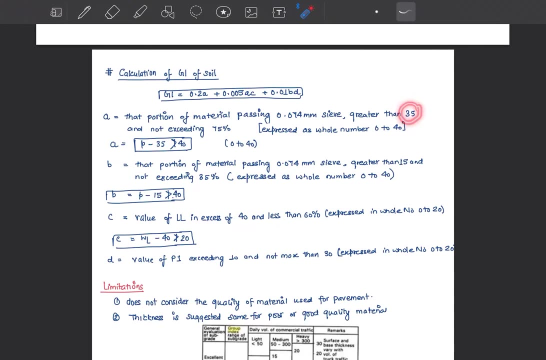 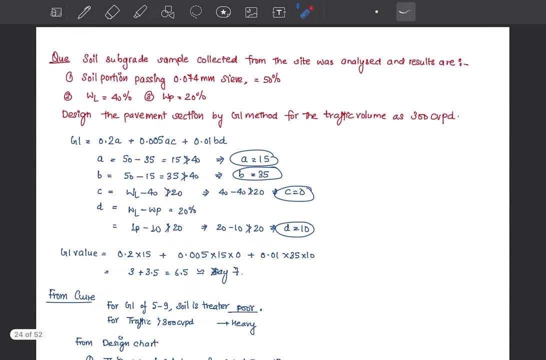 Now what was A? A is the portion of material which is passing 0.074 mm sieve. If you look at the theory that portion of material passing 0.074 mm sieve greater than 35 but not exceeding 75%, So greater than 35% but not exceeding 75.. 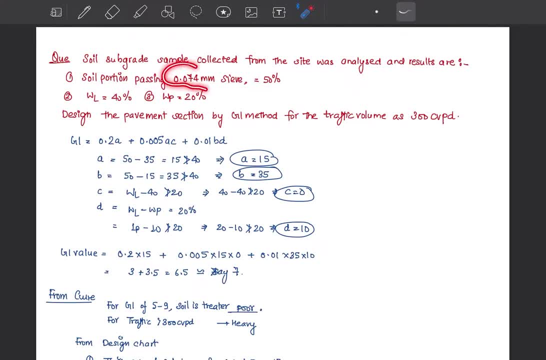 So how much more than 35 is A? So we have A. We have given that we are passing 50% from 0.074 mm sieve, So what will be A? How much more than 35%? So 50 minus 35.. 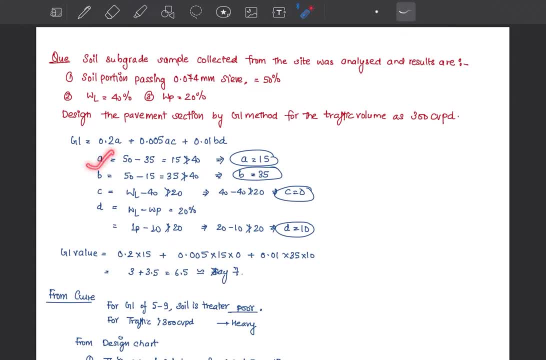 So this would be 15%. So the value of A that we have got is 15 and we express this in the whole number range of 0 to 40. So 15 is not more than 40, it means 15 is accepted. 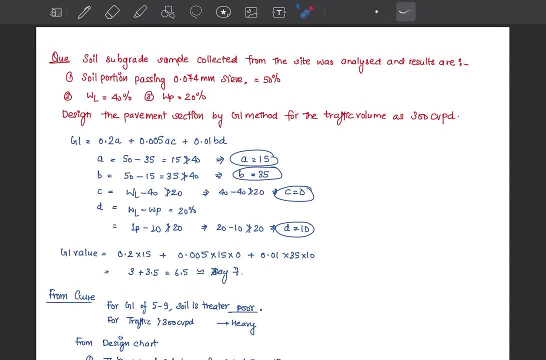 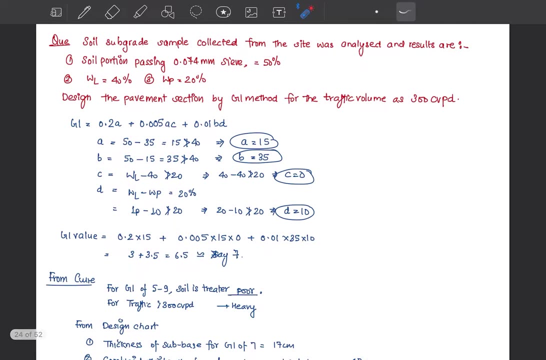 So what is the value of A 15.. What is B? B is the soil portion passing 0.074 mm sieve which is not exceeding 15%, which is greater than 15% and not exceeding 35%. So here you can see that we have 50%. so how much more than 50, 15%. 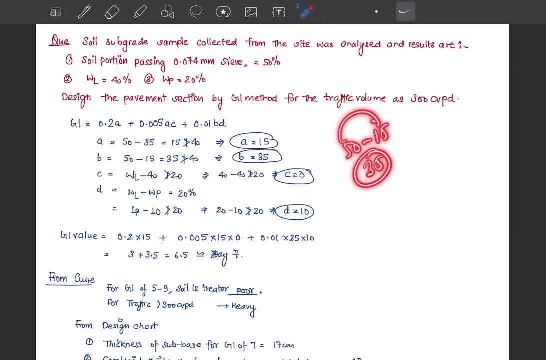 So how much more than 50 minus 35?? Now it is 35. But we know that it should not be more than 40. So here our value is in the range of 0 to 40.. So the value of B is also in the range of 0 to 40.. 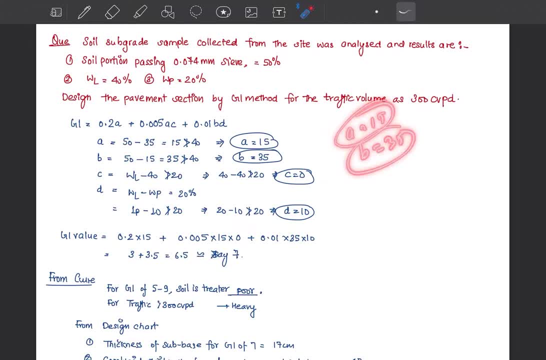 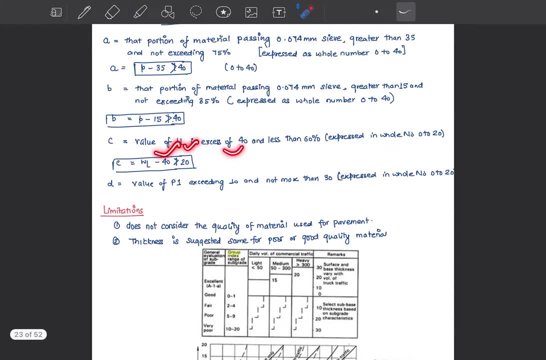 So how much more than 40? It is 35. So we have got A as 15 and B as 35.. Now what is C? C is the liquid value of liquid limit in the axis of 40 and less than 60.. 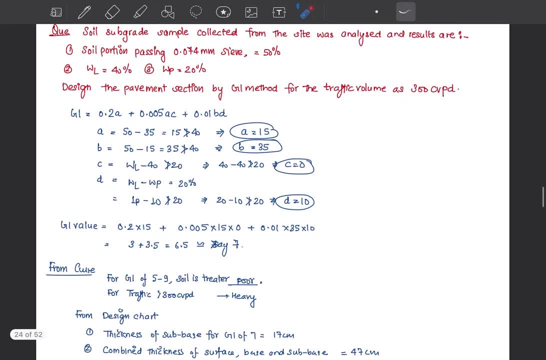 So basically, the liquid limit will lie in the range of 40 to 60.. So now, what is the liquid limit here? 40% is given. So how much more than 40 is the liquid limit? So 40 minus 40 is basically 0.. 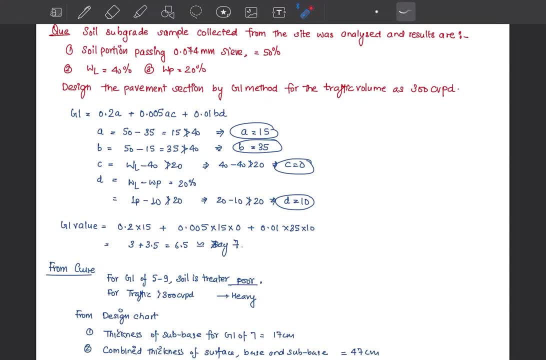 So what is the value of C? It will be 0.. What is D? D is the same. The plasticity index should be in the range of 10 to 30. So how much more than 10?? Now we have to find the plasticity index. 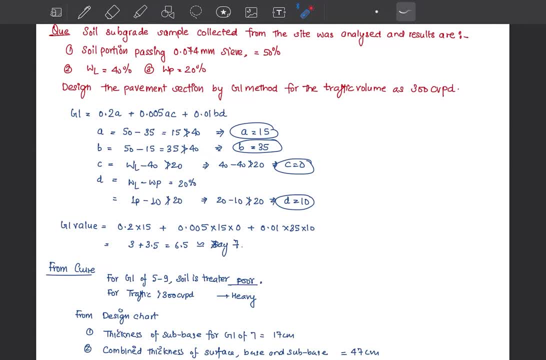 So how will we find the plasticity index WL minus WP? So the liquid limit is given as 40% WL and WP are given as 20%. So how much is the plasticity index 20%? So what does D say? 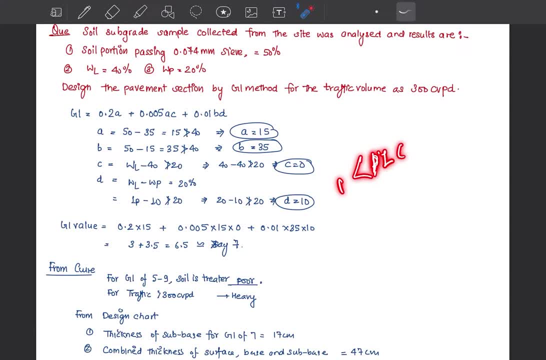 The plasticity index should be in the range of 10 to 30. So it should be more than 10 and less than 30. So how much more than 10?? 20.. So how much more than 10? 20 minus 10 is 10.. 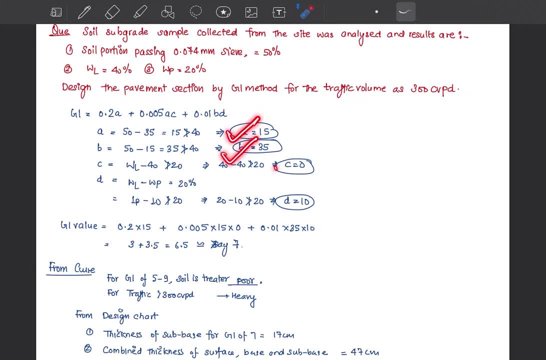 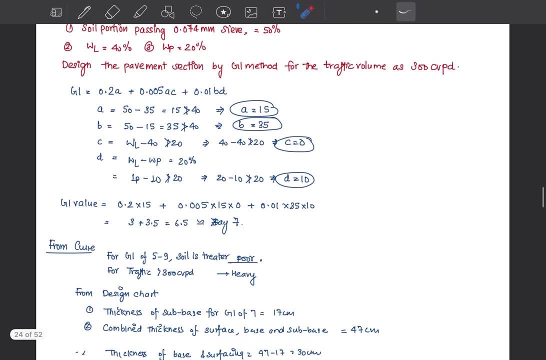 So what is the value of D? 10.. So A is 15.. B is 35.. C is 0.. D is 10.. Now let's put the values of A, B, C and D in the standard equation. 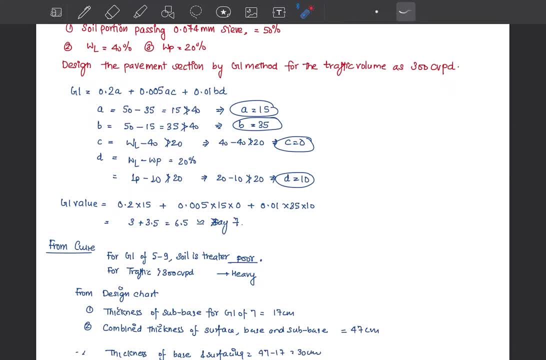 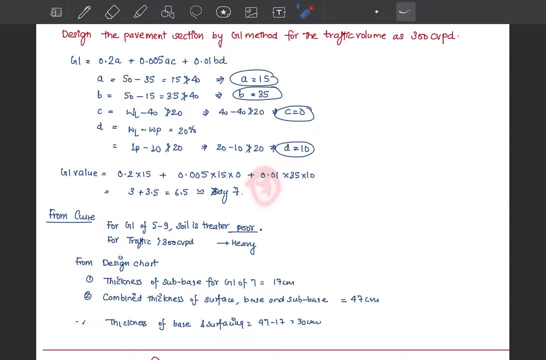 So in this equation, when we put it, we got the value of GI as 6.5.. Let us say in the round figure we consider it as 7.. So we got the GI value as 7.. Now we know that from the design curve. 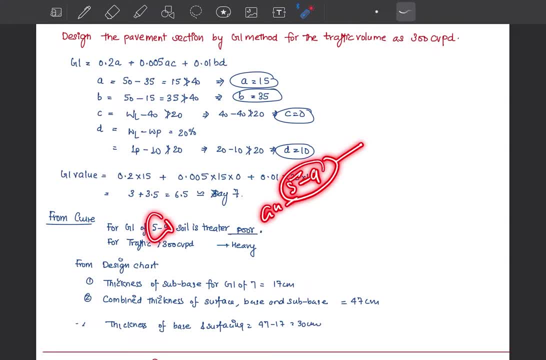 the soil between 5 to 9, the GI value. we consider it as poor soil But that is nevertheless of our discussion. But our main topic is that we should know the GI value. So we got the GI value as 7.. 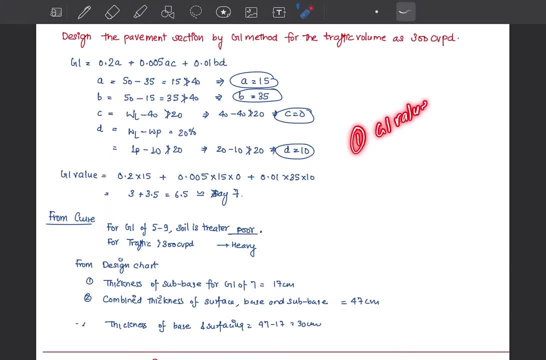 We calculated it. Now what is the second step? The first step was to calculate the GI value. The second step is to do traffic categorization. Okay, So look at the question. The traffic is 300 CVPD, That is, 300 commercial vehicles per day. 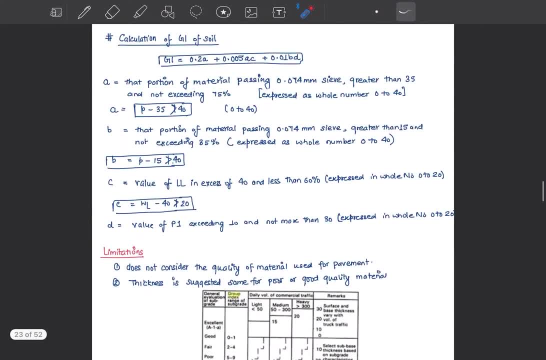 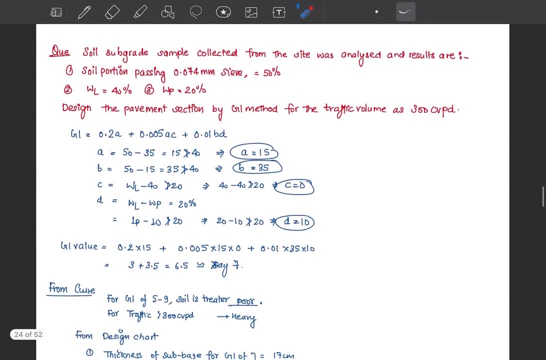 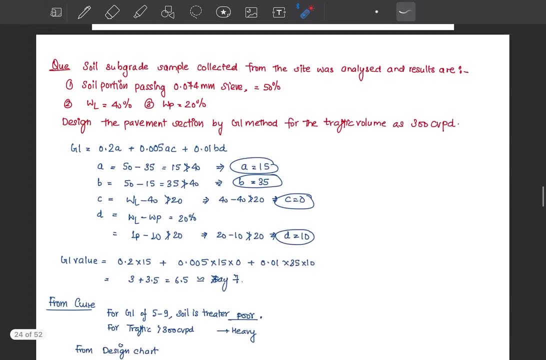 So if we look at the design curve, so when we read the theory- so greater than 300- we used to consider heavy traffic. Okay, So the traffic here is heavy traffic. Okay, Now we will refer to the design chart. Okay, 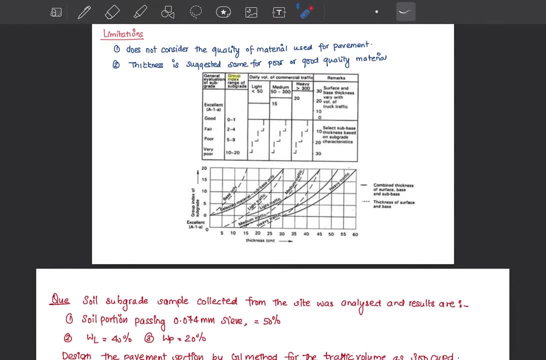 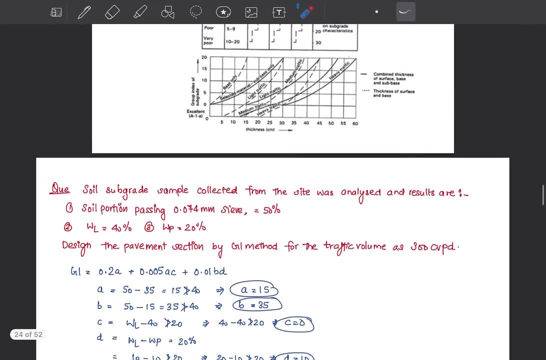 Let's go So if this is our design chart, Okay. So let's talk about the group index value of 5 to 9.. Okay Means in the range of group index of 7.. So for 7, our thickness would be ranging between 10 to 20.. 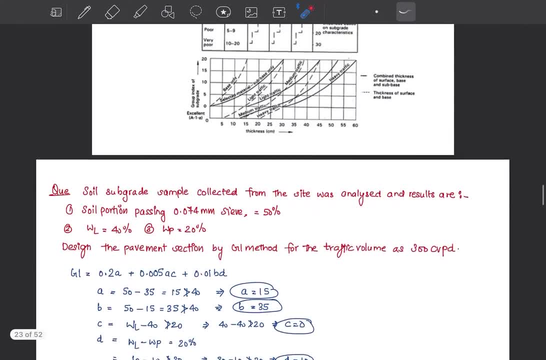 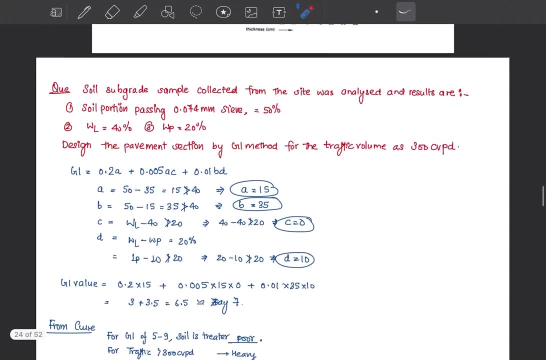 Okay, So between 5 to 9.. So how much will it be for 7?? Approximately, by interpolation you can see that the value will be 17 centimeters. Okay, Whereas if you look at the second curve for the combined thickness, 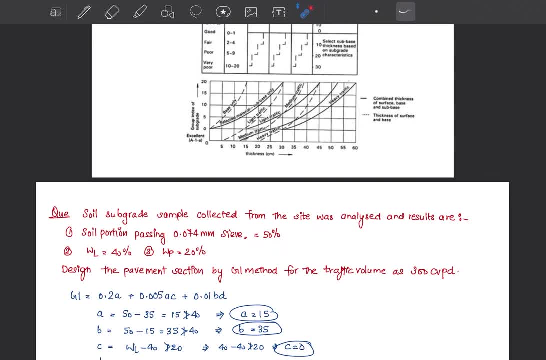 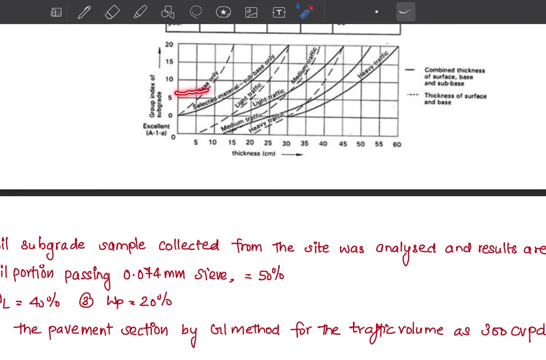 then look at the combined thickness, We have heavy traffic. Okay, Basically, this is your heavy traffic. Okay, And what is our group index value? 7.. So 7 and heavy traffic. So somehow the value will be colliding here. 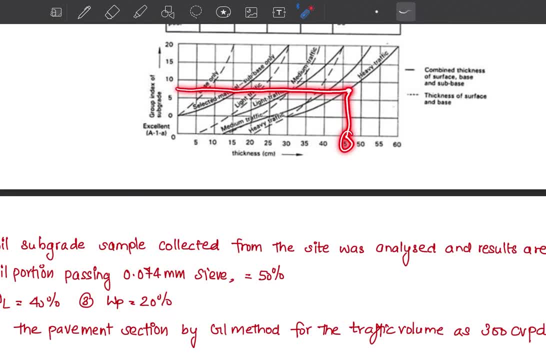 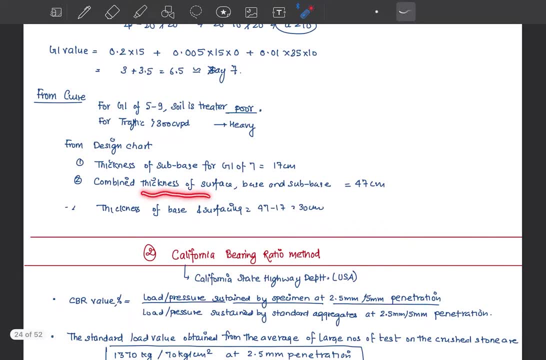 Okay, So the value that will come here for the group index value of 7, this will be near about 47 centimeters. Okay, So that is why the combined thickness of the surface base course and sub-base course is 47 centimeters. 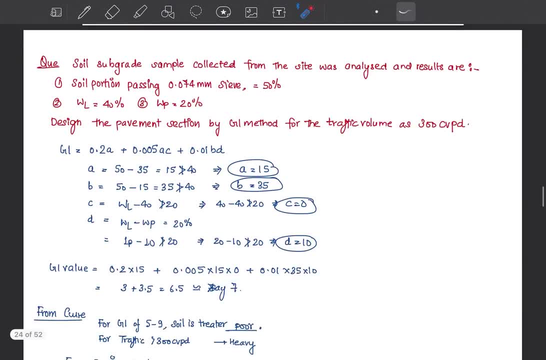 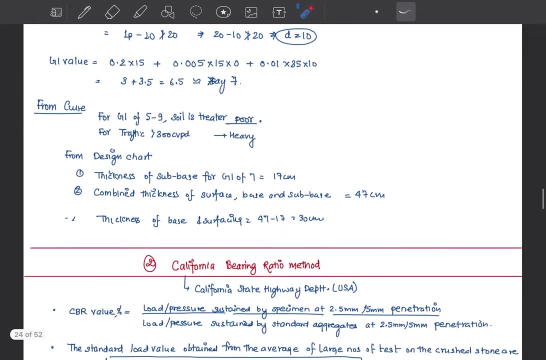 So the total combined thickness given to us, from which the sub-base was given a separate table. Okay, This was 17 centimeters. Okay, So our sub-base was taken out, So we can take out the base course and the surfacing course. 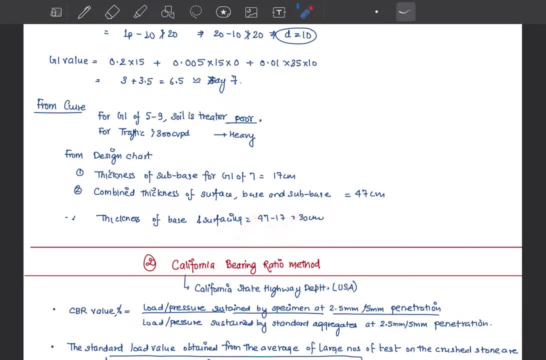 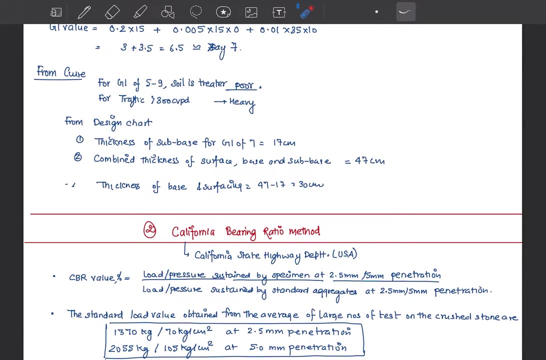 From the total we have minused the sub-base, So we got the thickness of the base course and the surfacing course. So in this way we do the payment design with the group index method. Okay, Payment design basically means the payment thickness requirements. 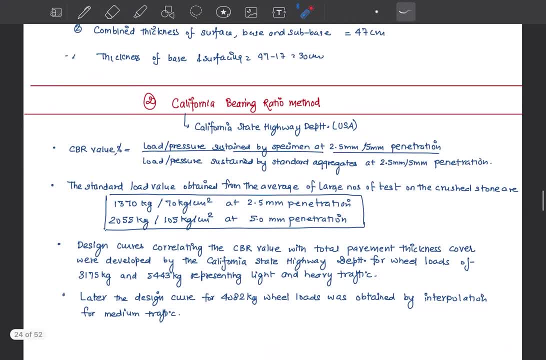 The thickness requirement of the different layers. Calculate that Okay. Now let's move on to the second method, empirical method, that is, CBR method, California Bearing Ratio method, Though in the transportation engineering you have already studied about the CBR test in detail. 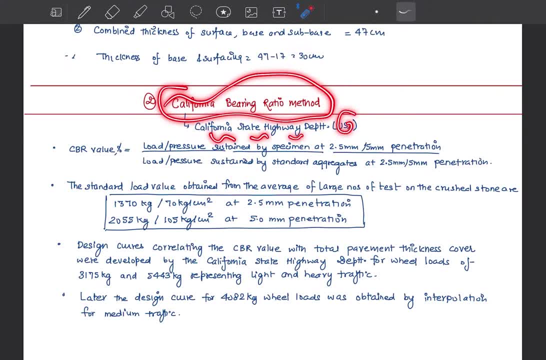 Okay. This method was developed by the California State Highway Department of USA, where he has given a relation to calculate the CBR value. How do we calculate the CBR value? This is the ratio of the load sustained by a specimen at 2.5 or 5 mm penetration. 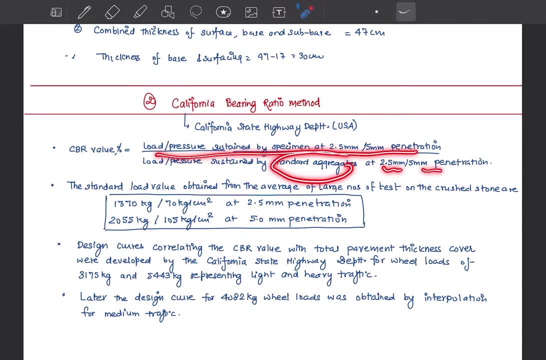 upon the load sustained by the standard aggregate at 2.5 and 5 mm penetration. So basically, between 2.5 mm and 5 mm penetration. we calculate the ratio of the load sustained between a given sample and a standard loading. 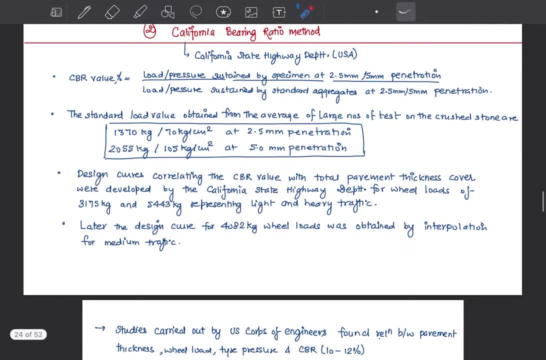 Okay, And what are the standard load values? Okay, So the standard load value has been recommended, So 1370 kg. And if we talk about 70 kg per centimeter square at 2.5 mm of penetration level, 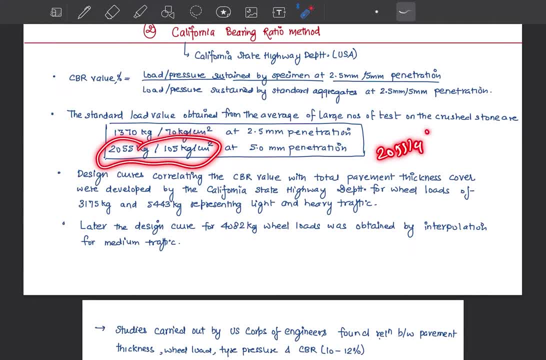 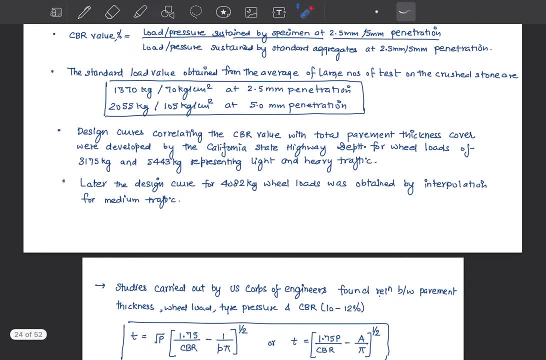 whereas at 5 mm of penetration the value recommended are 2055 kg and 105 kg per centimeter square. Okay. On the basis of various tests, we found that the CBR values with the total pavement thickness cover were developed by the California State Highway Department. 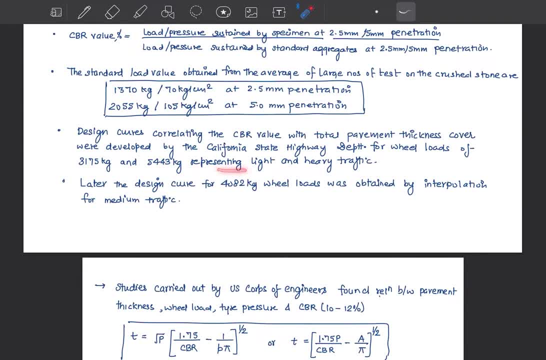 for wheel loads of 3175 kg and 5443 kg, representing light and heavy traffic. So, basically, your California State Highway Department designed a curve. Okay, They designed a wheel load of 3175 kg and 5443 kg, which basically represents 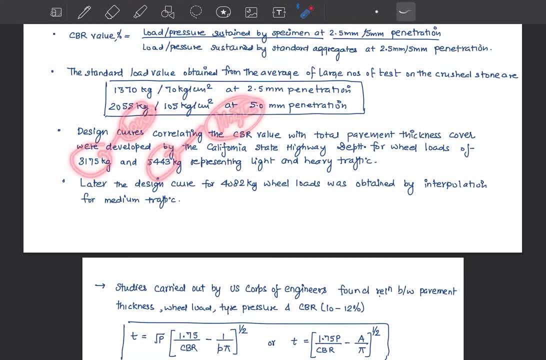 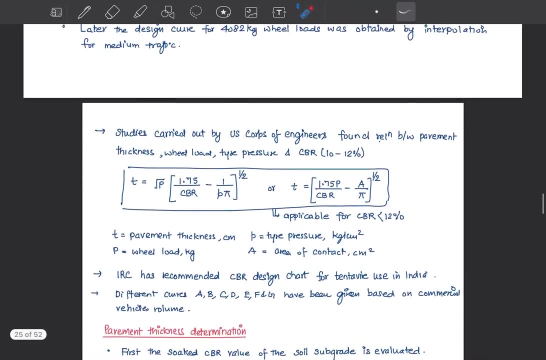 your low traffic And this representing the higher traffic. Okay, So for lower and higher traffic, they plotted a curve, Okay, And from that curve they gave the values for the medium wheel loads by interpolation, which is in the middle, Okay, 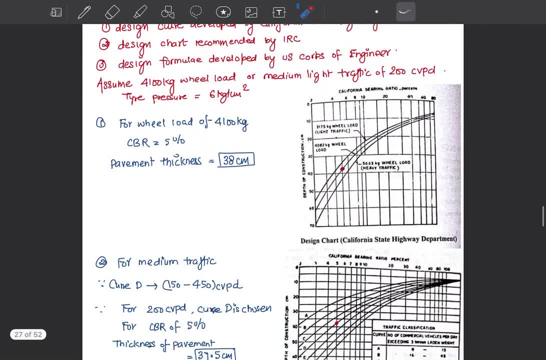 You can see in this question. Yeah, This is the design chart which was recommended by the California State Highway Department. California State Highway Department. you can see that they have given the chart basically on the basis of California CBR value percentage and for the different loading, how much wheel? 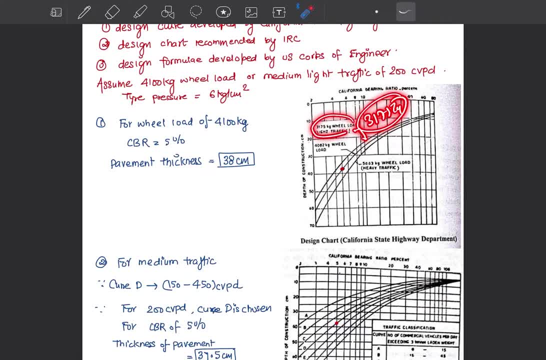 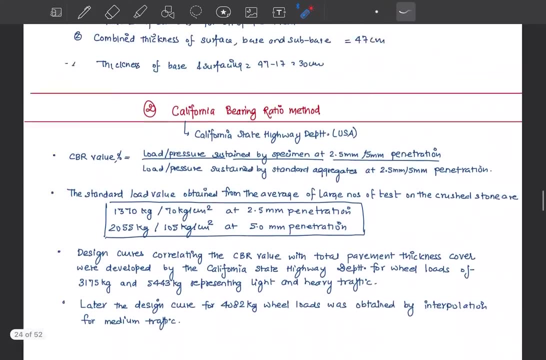 load is coming. if this is your 3175 kg, this is for the light traffic and this is for the heavy traffic and for the semi-tunnel, they have interpolated the design curve for medium traffic. they have chosen the design curve. okay, so we were talking that the US Corps. 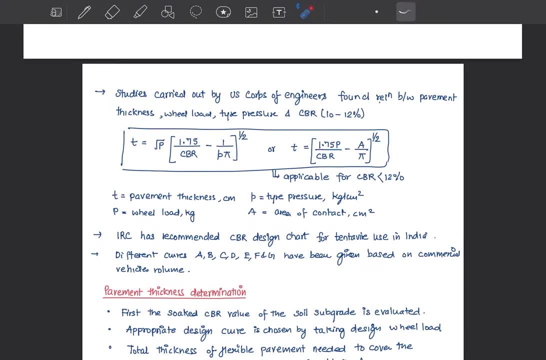 of Engineers. they also gave a relation related to the CBR test. okay, what relation did they give that? how can we calculate the pavement thickness? they gave a relation of pavement thickness which was based upon the wheel load, tire pressure and the CBR value. okay, the 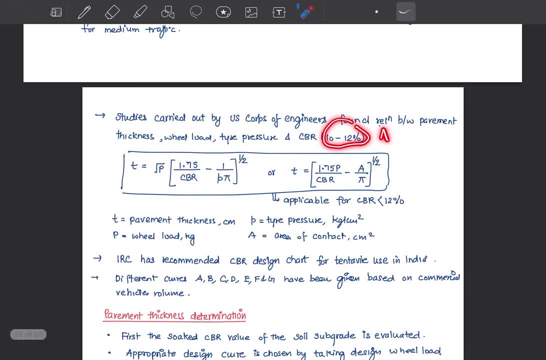 CBR value. this formula, what he has given, Was valid for the CBR range of 10 to 12%. however, the formula which was given was applicable up to CBR value of 12%. the formula which was given as T is equals to under root of. 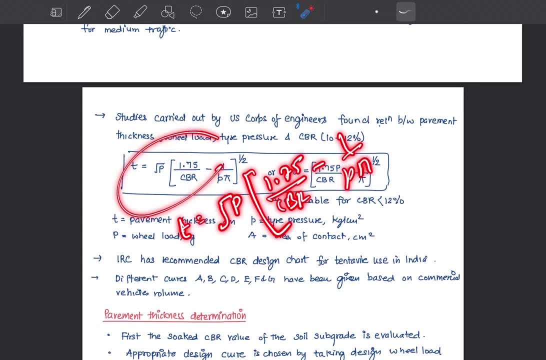 P1.75 upon CBR minus 1 upon P5 to the power over 2,. however, you can modify your formula according to your convenience, so sometimes this formula may be used. sometimes this formula may be used as far as the data is given in the question. 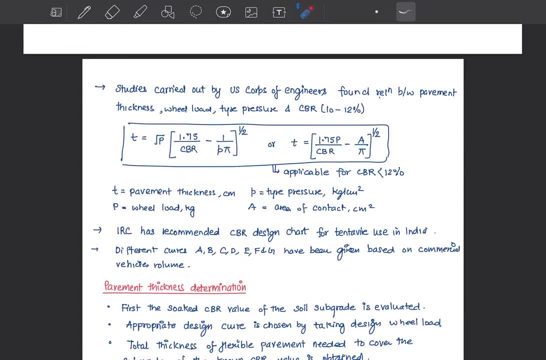 Okay, And what is T? T is the pavement thickness, which is in centimeter. what is P? P is the wheel load, okay, in kg. what is small? p? this is tire pressure, kilogram per centimeter square. what is A? A is the area of contact in centimeter square. okay, this was the method. 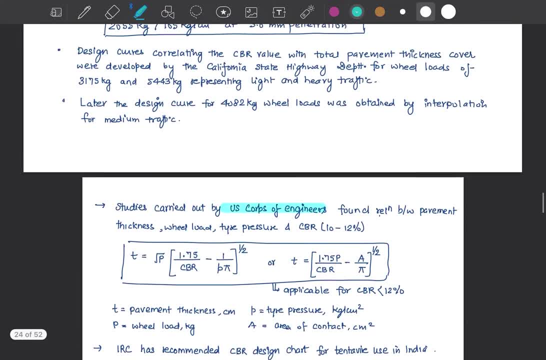 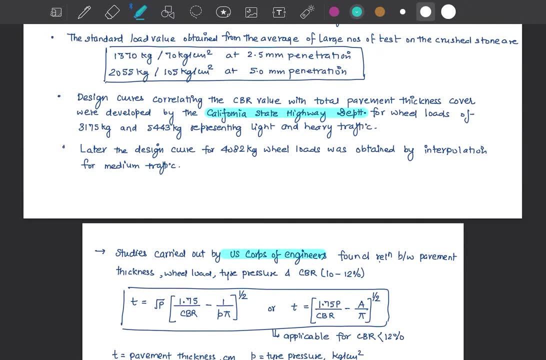 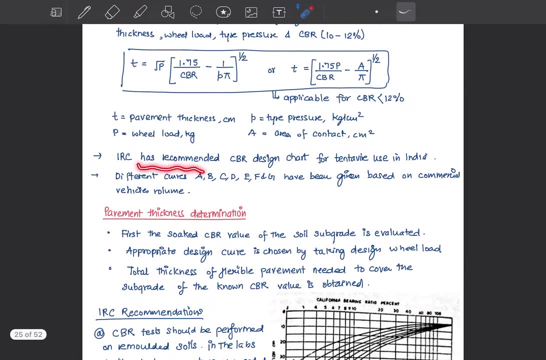 which was given by the US Corps of Engineers. okay, So three methods. The methods were there. okay, one was of California State Highway Department, one was of US Corps of Engineers, which gave its method. okay. Now IRC has recommended CBR design chart for the tentative use of India. okay, IRC. 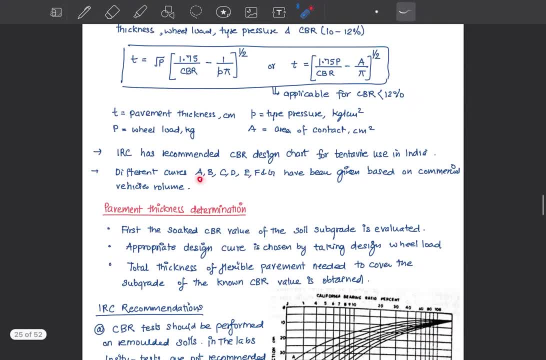 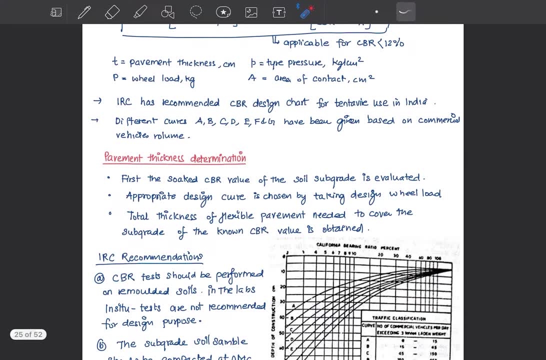 gave its method that they gave different design charts- okay, and gave different curves- A, B, C, D, E, F- on the basis of commercial vehicle traffic. okay. Now how to determine the pavement thickness? People do this right. 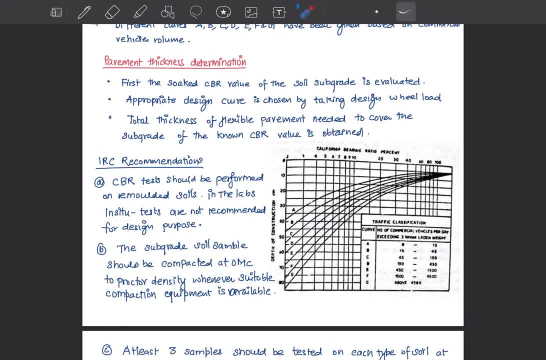 So the first step is to soak the CBR values, the soilsamp, to soak for 4 to five days right, And then after that the CBR values are evaluated by the soilsab. How to evaluate the CBR values, we have already covered in Transportation Engineering. okay. 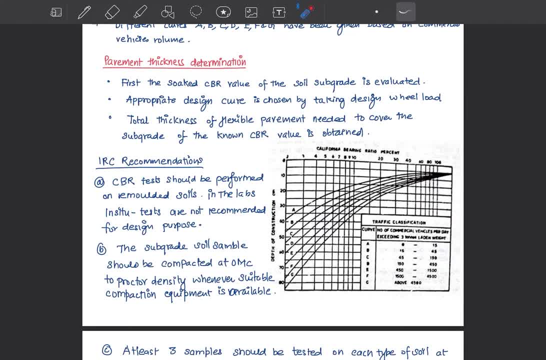 We will calculate the CBR value on 2.5mm and 5mm penetration right Then. after that, we choose the design curve. okay, The design curve is okay. So we will understand. okay, Okay, Okay. 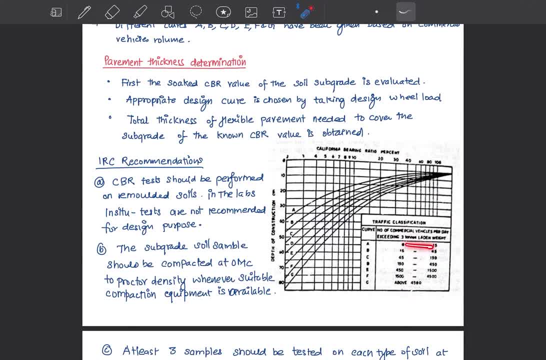 according to which we will choose the design curve. let us say that: how much is your design traffic? according to which this design curve is given: A, B, C, D, E, F, G. these curves have been suggested. on the basis of these curves, we select the values. okay, total thickness. 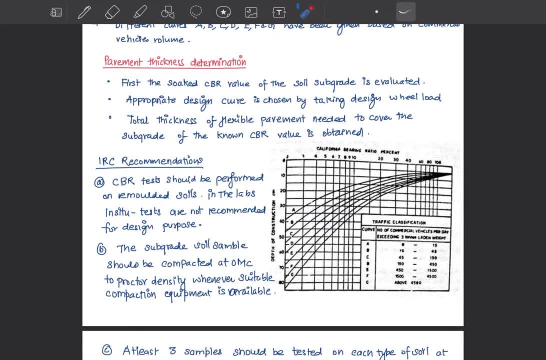 of the flexible payment needed to cover the subgrade of the known subware is obtained. so, basically, on the basis of the CBR value, we and on the basis of the design curve which we need to follow, we just predict the total thickness of the payment which is needed to. 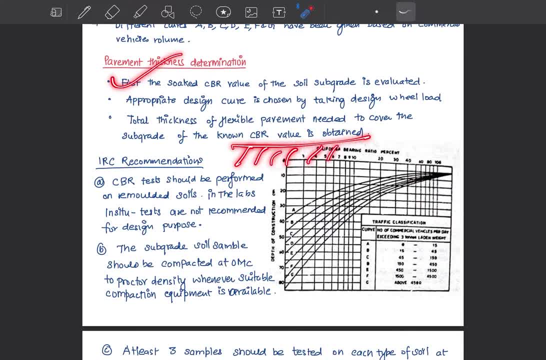 cover the subgrade. so basically, in this method we will select above the CBR value. let us say this is subgrade. okay, so the values that will come here in this curve. let us say that the value that is for our CBR has five percent. if we are choosing this, then 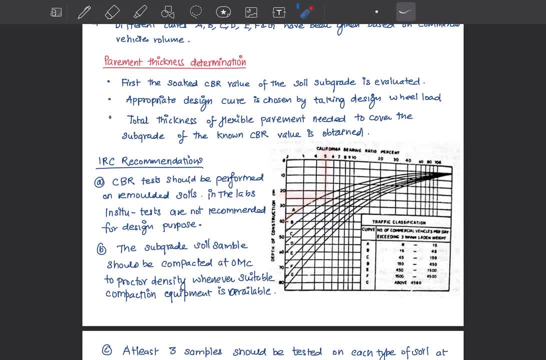 it will come here. value, let us say it is coinciding. then we will say that on the subgrade: if this is our subgrade, then on the subgrade, our layer of 22 cm is required. ok, so basically on. 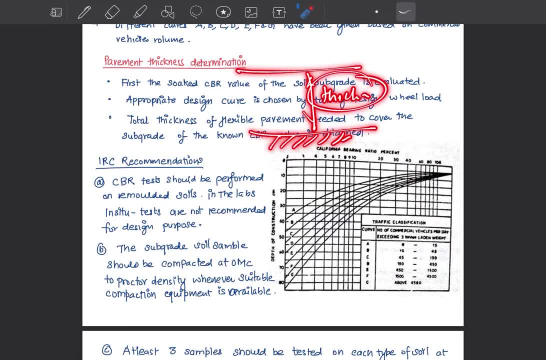 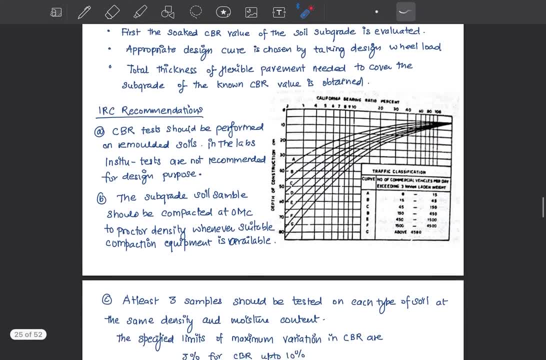 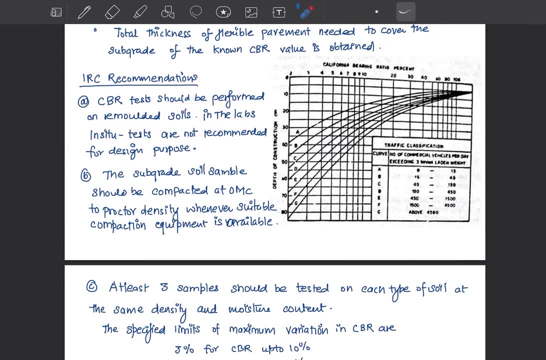 the subgrade, how much thickness of layer is required. this method is told by the CBR method. ok, so IRC also had some recommendations for this method. what are those recommendations? that is, CBR test should be performed on remolded soil in the labs, so this CBR test should. 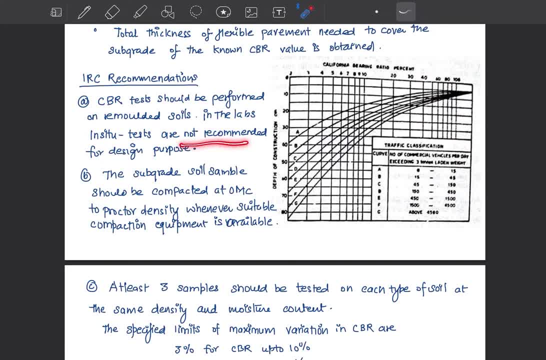 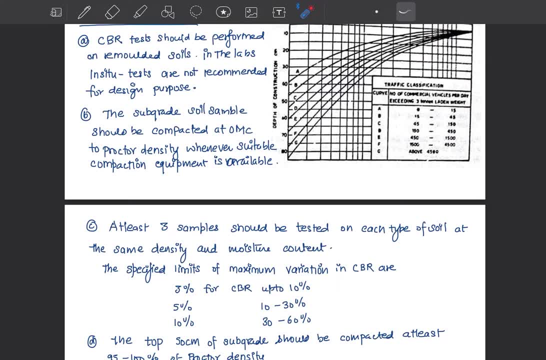 be performed in the remolded soils in the lab. in-situ tests are not recommended for the design purpose, so site tests are not recommended. the soil subgrade sample should be compacted at optimum moisture content to practical density whenever suitable compaction. 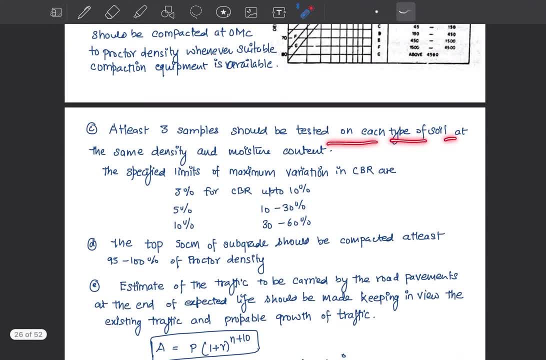 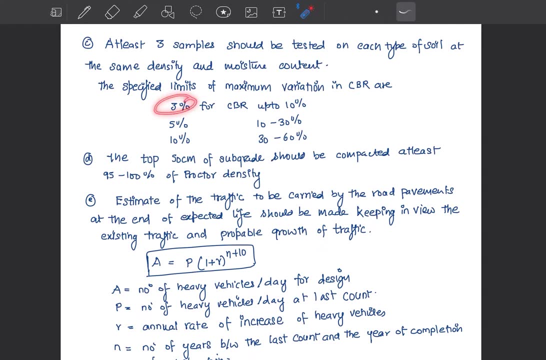 equipment is available. at least three samples should be tested on each type of soil. so we will do testing of at least three samples, ok. for each type of soil at the same density and moisture content. the maximum variation that is allowed in CBR values is allowed. up to 10%, 10 to 30%, 30 to 60% of CBR variation is allowed. ok, the top 50 cm of the subgrade sample should be compacted at least 95% to 100% of the proctored density. so the top. 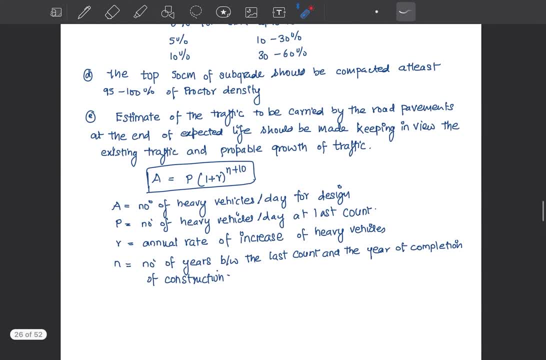 50 cm layer of the subgrade should be well compacted to 95% to 100% of proctored density. the traffic estimation estimate of the traffic is to be carried out by the road pavements at the end of the expected life should be made, keeping in view the existing traffic. 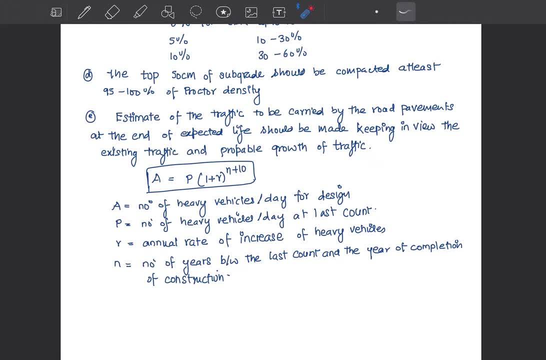 and the probable growth of traffic. so basically, how much traffic is going to come. we are calculating the expected traffic. so basically, how much traffic is going to come. we are calculating based on your existing traffic and on the basis of probable growth of traffic. 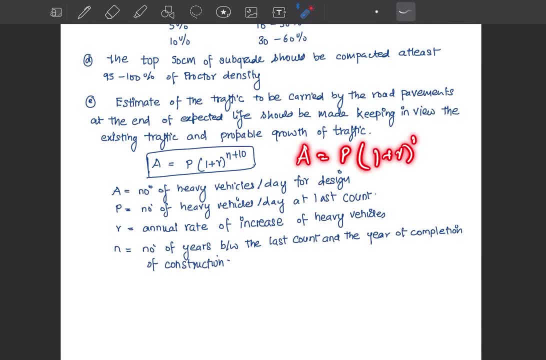 by using this expression. so A is given as P into 1 plus R, to the power n plus 10,. what is A is the number of heavy vehicles which has to be chosen for the design. ok, our expected traffic is going to be this much. what is P? P is the number of heavy vehicles. at last. 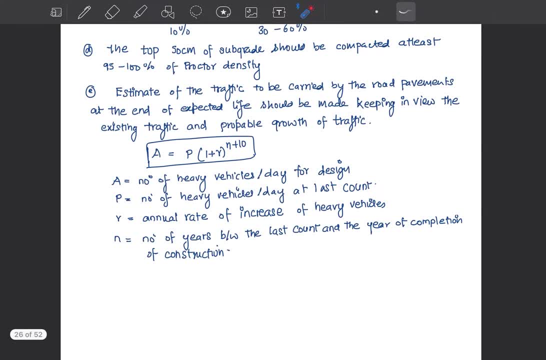 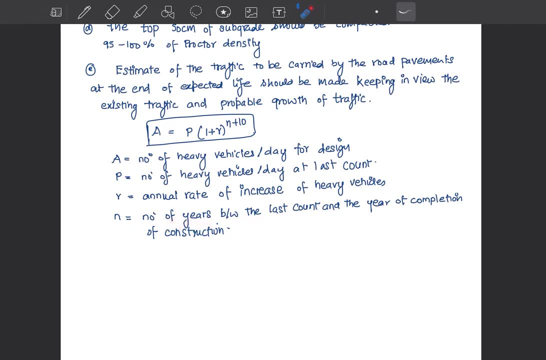 count, which is our last count, or basically present, where we have taken the reading. ok, what is R? R is the annual rate of increase of heavy vehicles, n is the number of years between the last count and the year of completion of construction. ok, when we have done last. 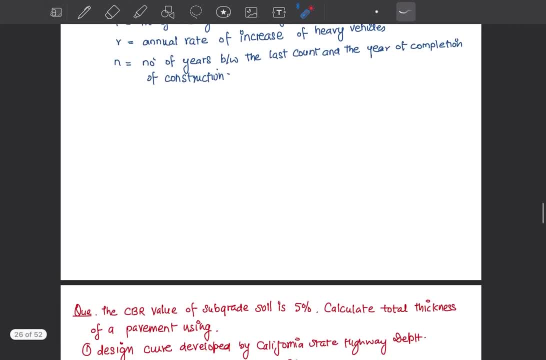 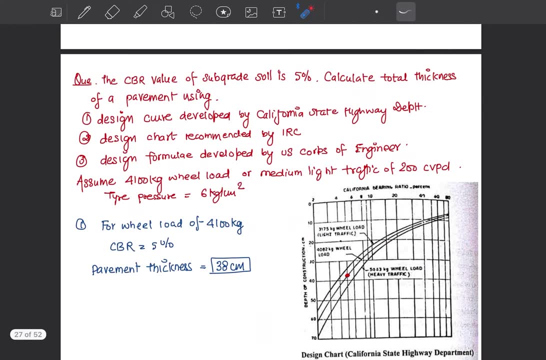 count how much time has it taken in the construction period? that is n. ok, now let's take numericals to make this theory very clear. The first question relates with the CBR value of the subgrade soil. is 5%? calculate the. 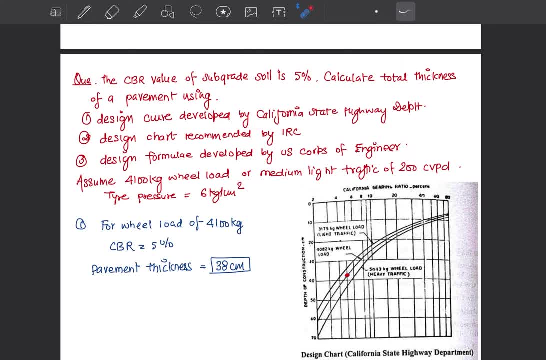 total thickness of the subgrade soil. The payment using design curve developed by California State Highway Department. design chart recommended by IRC design formula developed by US Corps of Engineers. This is very important question because it will cover all the three methods as recommended. 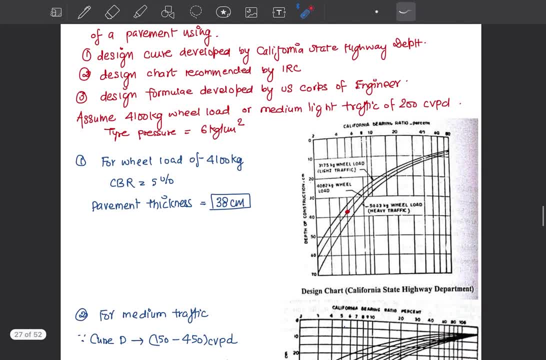 for the as related with the CBR test. ok, Also, there have been certain important data which has been given. Assume: 4100 kg wheel load or medium light traffic of 200 cvpd. Ok, tire pressure of six kilogram per centimeter square. okay, now let's move on to first question. 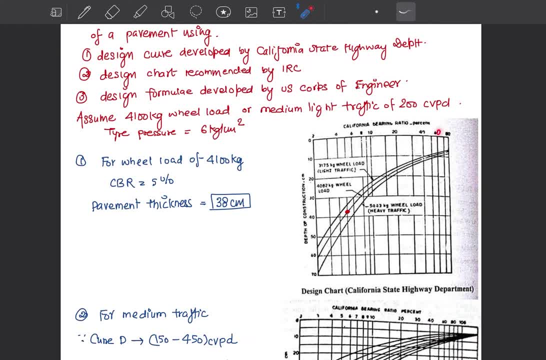 that is the design curve developed by the california state highway department. so, looking at the design curve which have been given, as for the california state highway department, they have given this chart. okay, now in question, we have given data, we have given cbr value: 5 percent. 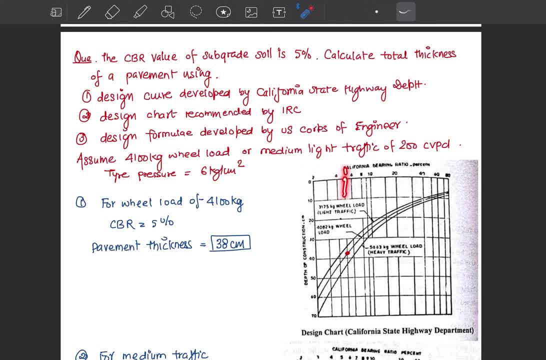 okay, let's consider the cbr value of 5 percent. okay, so this cbr value is 5 percent. so this One curve is to be chosen. plus now we have We load question of 4,100 kg. so see this, looking at a crowd of 408 one. it is the second crevice of carасти, medium ey. that would be. 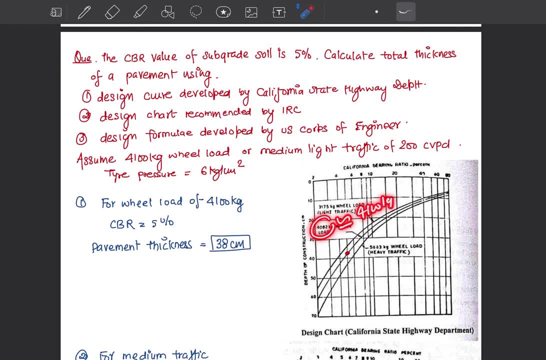 applicable in our case. ok, so re two is approximately equal to four TV 100 kg. ok, so from our medium curve is given As a picture. the unevenness will have clothes in which sovereign meaning cannot be saw in the комнаt. so the bound is given and, ah, that division is not important. 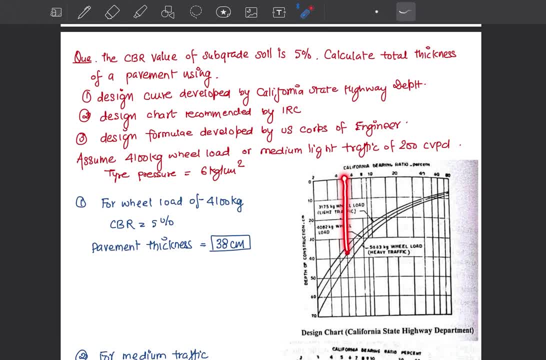 at that distance the thickness will be known, says by the distance Individually, the middle that would be valid. take the CBR range of 5% and the medium curve. tom loki a value. jo hai a coincide curry. take it to y'all pay a value. okay, a red red say. 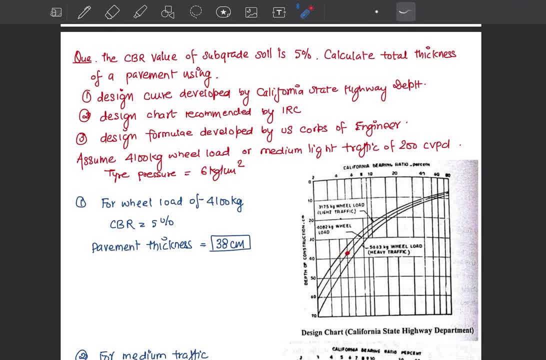 you many mark here that is coinciding. so basically, I put your payment thickness. are looking at the curve. can we say like this: the payment thickness requirement is your, your 38 centimeter. okay, this is for the method as developed by the California State Highway Department. okay, now let's move on to the design. 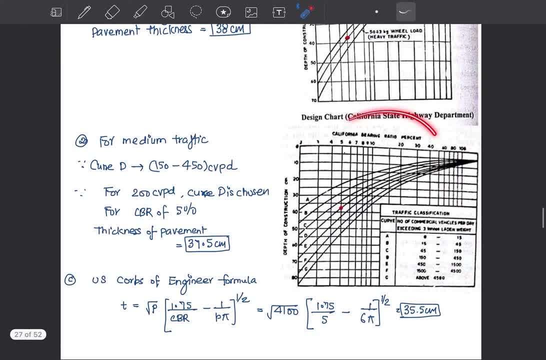 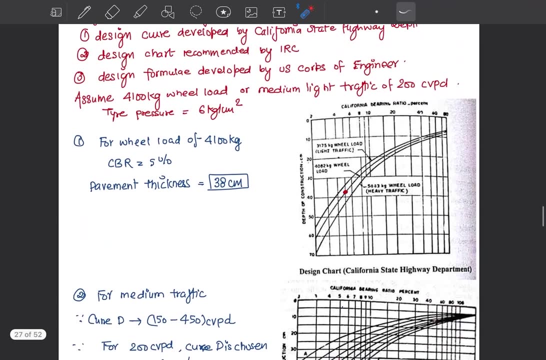 chart which was recommended by the IRC, okay. IRC has recommended a design chart based on the CBR value- okay. and on the traffic classification: take a kitna. traffic a whiskey according concert design charts were for: choose Karna ham logo: go. take a cushion media where a medium light traffic of 200 cvpd. take a. 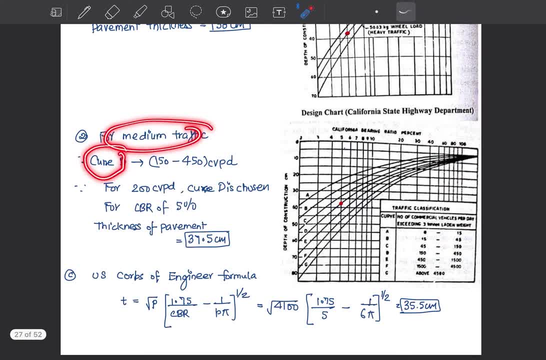 challenge. so medium traffic, amarra, kitna, hawa hai, karate ka to 150, sit for under 50 kg. too long. the look of the award: 200 CFD to 200 cvpd car. palavera 150 say 450, see them, 450 cvpd gab each Malayakara, so 150. 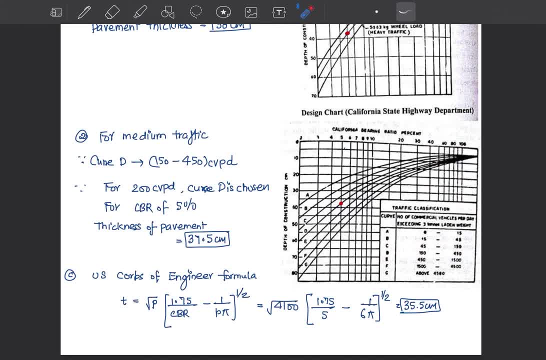 say for 50 kc VPD make on soccer wata have a sickly d car water. take Tom Lugo concert or which was gonna be curbs, was gonna to basically VR to choose the this curve d. okay, sorry, we have to choose the curve d. okay for cv 200. cvpd curve d is 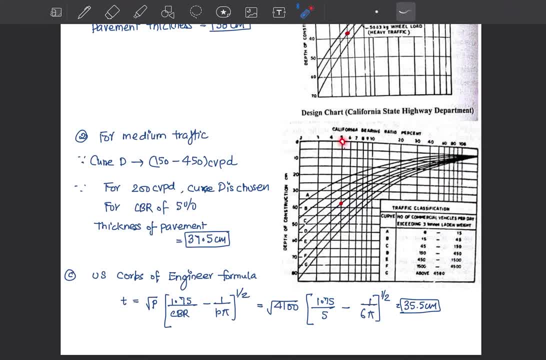 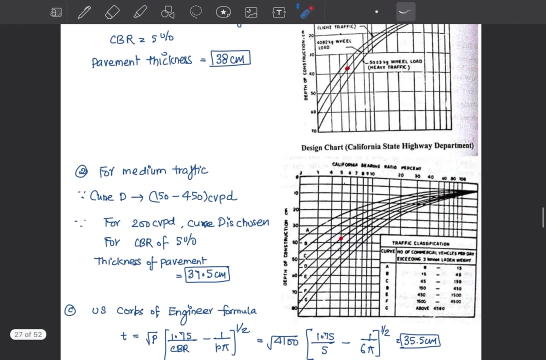 chosen for cbr value of five percent. okay. so we have given in the question cbr value of five percent and curve d is chosen, okay. so what is your our recommended thickness requirement? this is 30 here, 40 here, so it is near about here. so this is 37.5 centimeter. 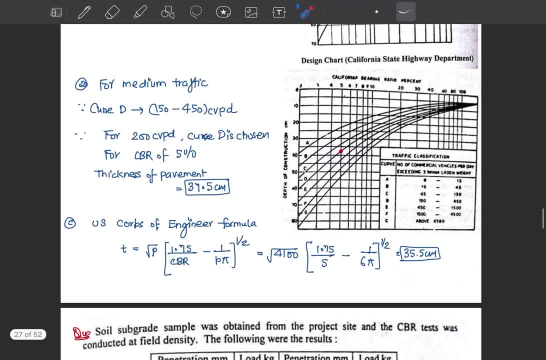 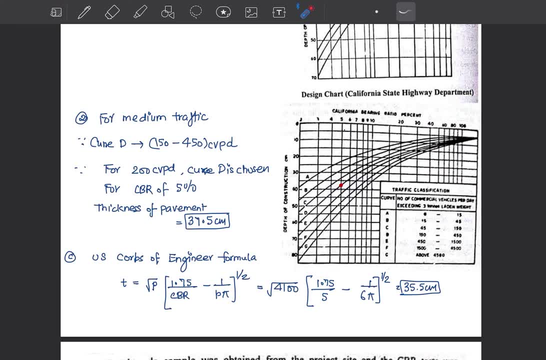 so you can see the result is somehow approximately related here. okay, now let's move on to the formula which was which was given by the us cops of engineer. okay, they have given the formula, that is: t is equals to under root of p, 1.7. 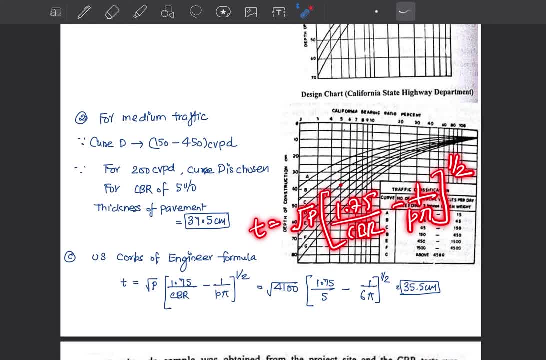 5 upon cvr by 1 upon p, pi to the power, 1 by 2 and using this formula, we know that design- this is design- wheel load, which is given as 4100 cbr value is given already in the question. five percent p is the tire pressure is already given, that is six kilogram per centimeter. 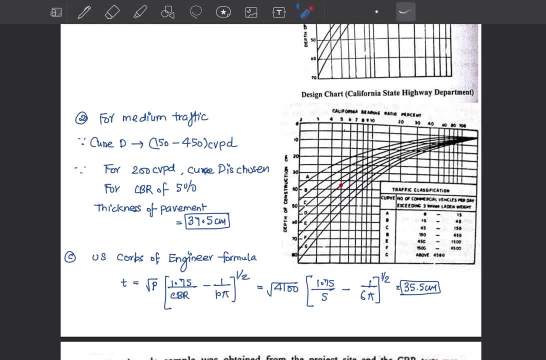 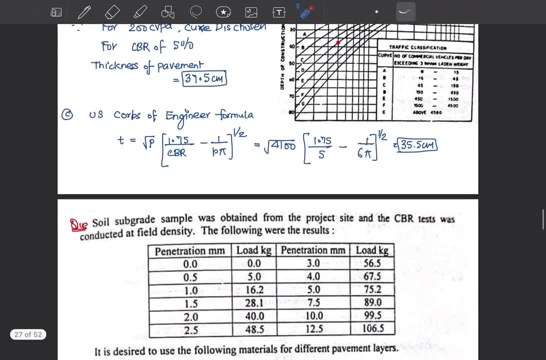 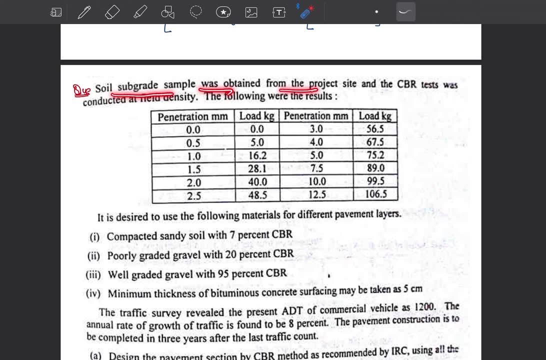 square, you will put all the values and you will get the payment thickness requirement as 35.5 centimeter. fine, now let's move on to second question. a soil subgrade sample was obtained from the project site and the cbr test was conducted at field density. the following test results were obtained: 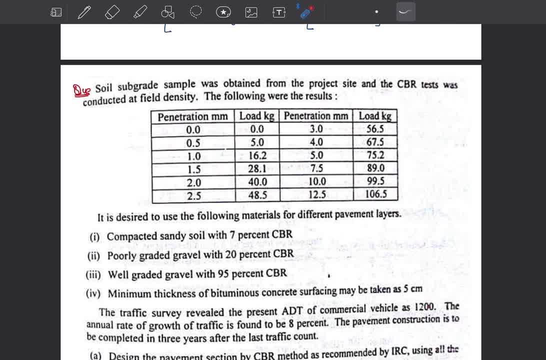 take at the different penetration level for different load values, with cbr testing. which of the calculate curtain will i take it? it is desired to use the following materials for the: 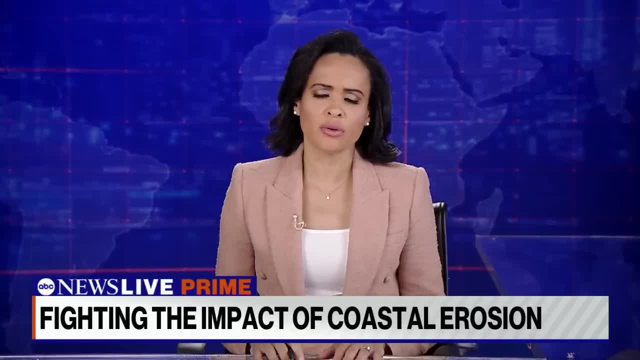 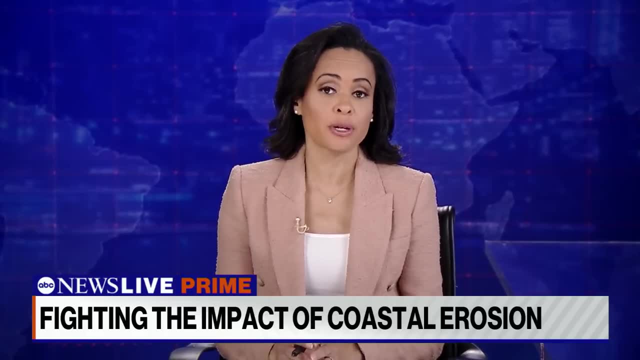 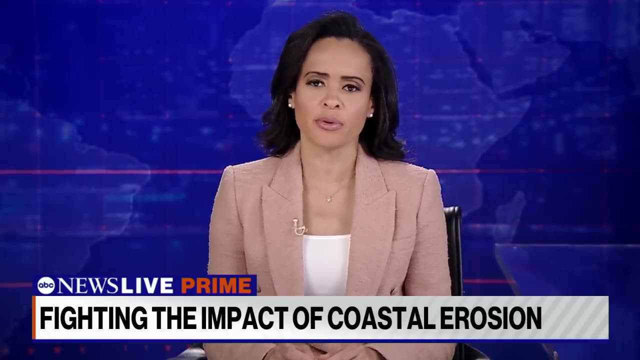 Tonight in Florida, residents are still picking up the pieces after Hurricane Nicole earlier this month and Ian earlier this year. All the storms are now long gone. The damage to our coastlines in some cases will be permanent. Can anything be done to save some of our country's most beautiful beaches? Chief Meteorologist Ginger Zee files this in-depth report.